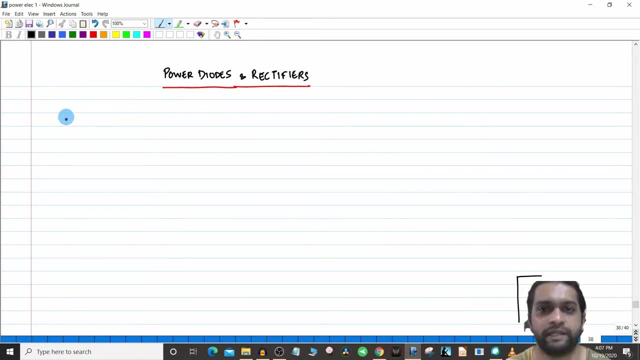 electronic device is basically a switch. Therefore the power diodes are also basically switches. So the diodes acts as switches to perform various functions. See, with various type of switching activities you get different type of applications. So they can be used as a rectifier, So they will be used in rectifiers and they can be used in freewheeling. 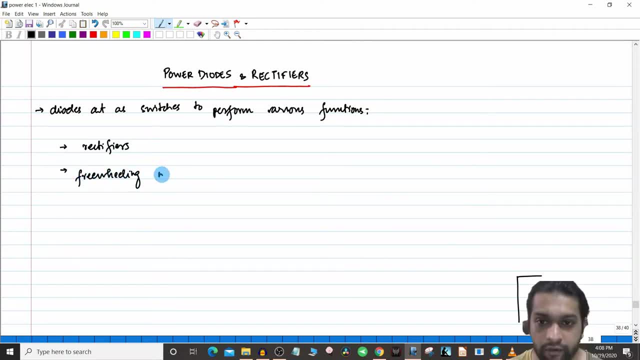 in regulator circuits. So we are just going through a broad list of applications: freewheeling in regulator circuits and then charge reversal in capacitors. That is, if you want to reverse the charge across the capacitors. charge reversal of capacitors: the switching action of the diodes can be used. 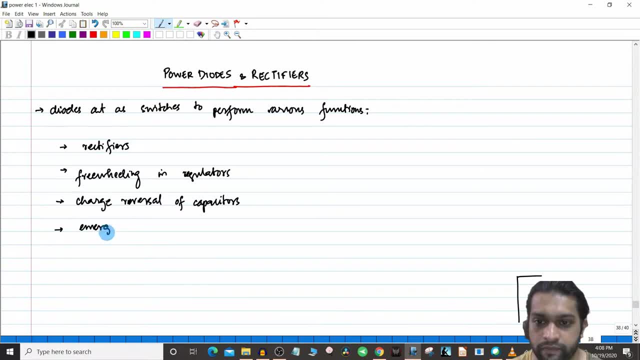 Other than that, then you are having the energy transfer between components. Energy transfer between components, So there the diodes are used. And then you are having another important application is voltage isolation. Voltage isolation: there diodes are used. We are just listing out these applications so that you can understand how wide 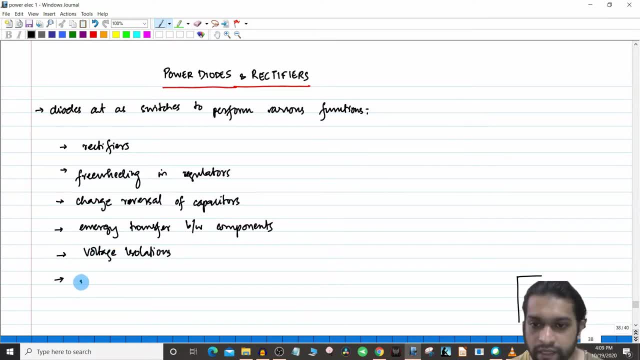 how wide spread applications of diodes are. Then energy feedback from source to load energy feedback from source to load such circuits diodes are used. Then, finally, you are having trapped energy recovery, trapped energy recovery. Okay, these are some wide areas of applications in which diodes are diodes and its switching. 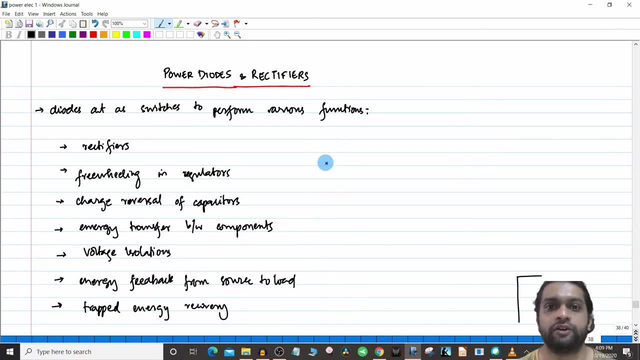 applications are used. Now the diodes that you must have seen in your colleges are the small diodes, right? So the small diodes usually cannot handle a lot of current Okay. So till now you might have seen your analog electronics lab etc. The small diodes like IN4001, 4148, etc. Now such diodes are 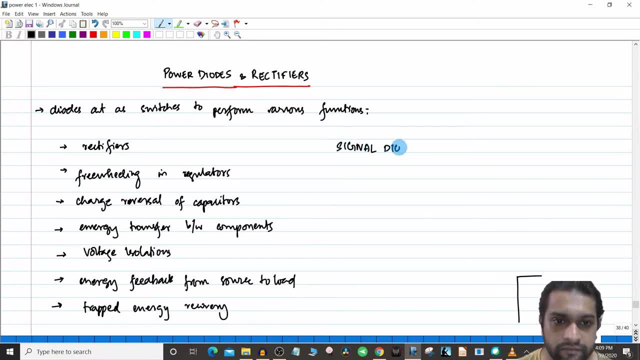 called signal diodes. okay, signal diodes, But we are not bothering about signal diodes, we are talking about power diodes. So the basic difference between a power diode and a signal diode is actually the power diodes. The difference between a power diode and a signal diode are about the same thing. 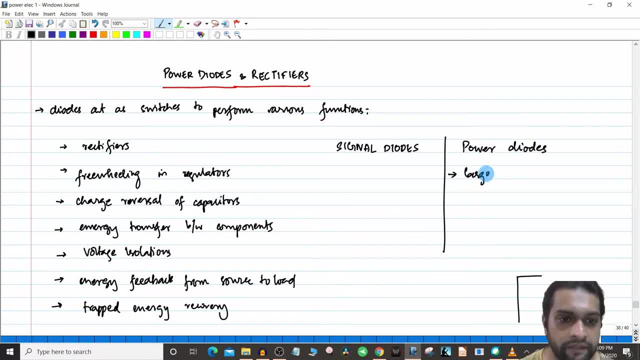 signal diode is that the power diodes have the larger current and voltage withstanding capability. But, however, the frequency response of power diodes is not as good as the signal diode. that is, the performance of the diode with a large spectrum of frequency is not. 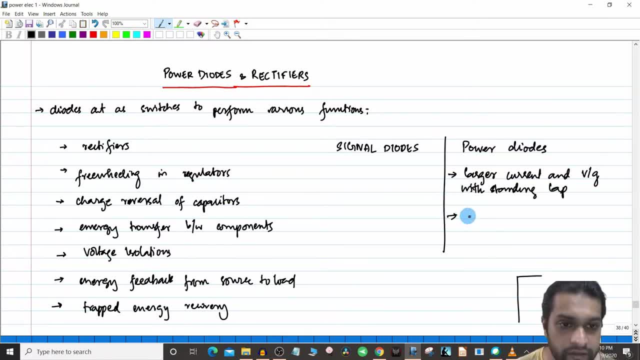 as good as the signal diode. So these are having frequency response is low. frequency response is low as compared to, as compared to signal devices, signal diodes. So I have just taken a simple data sheet here just to give you a comparison between these two. Now 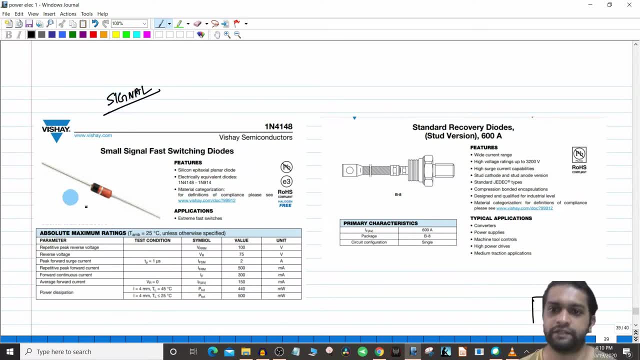 this is a signal diode, This is from Vishay semiconductors, a very popular manufacturer, and this is a power diode- Power diode. So if you can see the power diode here, you can see their ratings, can? I've just taken 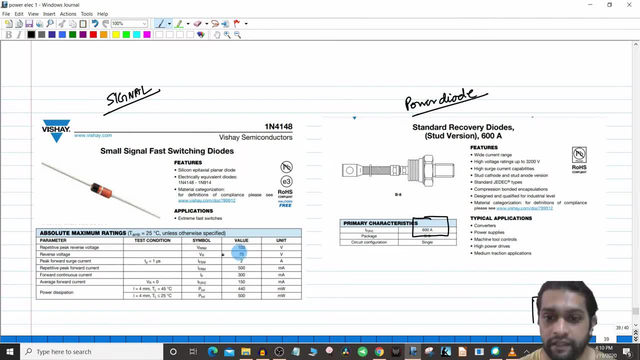 a random rating it can goes up to 600 amperes. huge rating here. if you see the ratings are comparatively. for example, if you see the forward continuous current it is 300 milli amperes. So usually the signal diodes are in that range, whereas the power diode you. 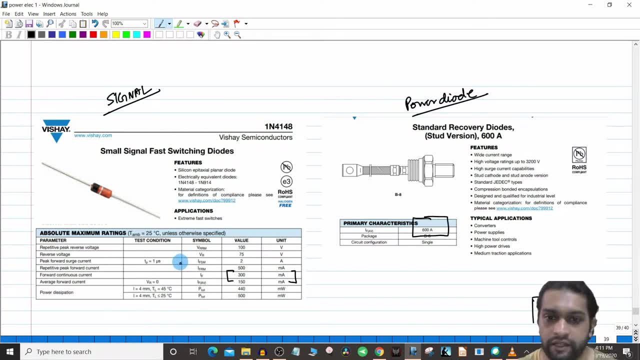 can find it in higher currents and higher voltage ratings. even if you see the peak forward, peak reverse voltage, voltage, if you see it is 100 volts. so these are not very high values. so this is a simple signal diode and this is the power you see, even the construction you see here. so this is the diode. 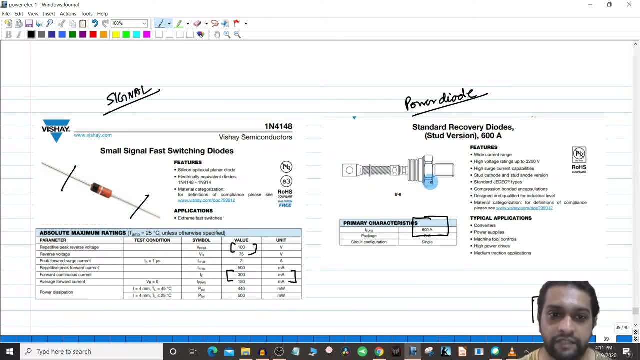 which you might have seen, but here you have the stud version where it is actually screwed type. so these are the uh diodes which you can see. see, you can. if you go to the website of a particular manufacturer you can find for various rating, 100 ampere, 200 and 300, 600 ampere. similarly here also. 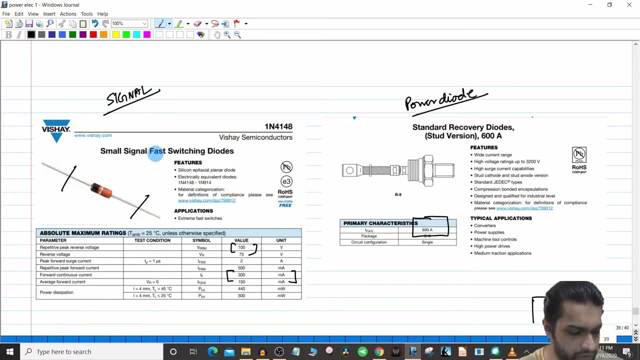 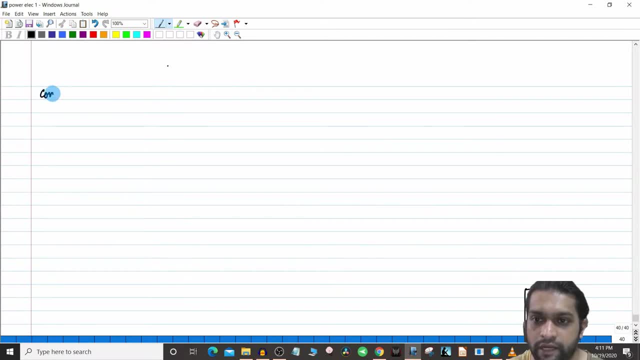 you can find a lot of different variations. now the commonly used semiconductors to manufacture these types of diodes, that is, the commonly used semiconductors- used semiconductors for the manufacture of power diodes are usually silicon, germanium or gallium arsenide. 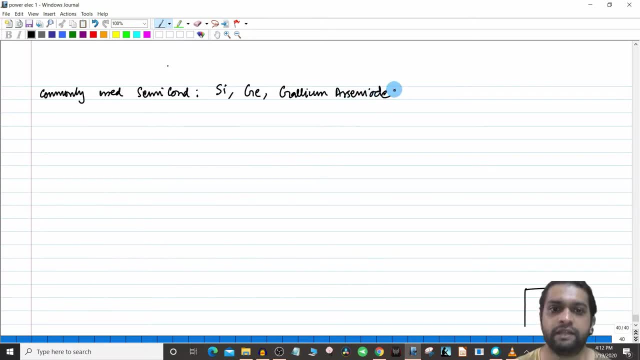 gallium arsenide. these are the popular choices which are available in the literature also. okay, so basically you know what is the type, what is the diode? the diode, i already told you it is that type of a device which has single pn junction. so here you are having your p type, n type material and 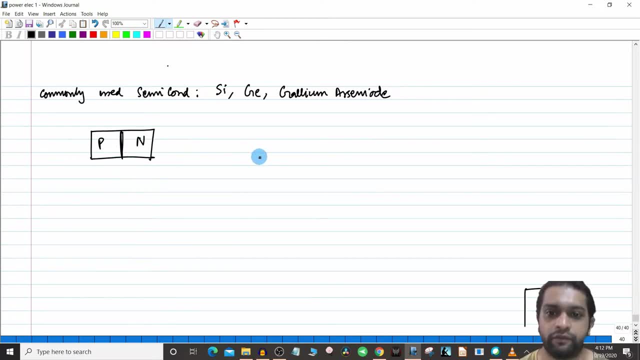 this is your diode right. so, schematically, if you draw the symbol of this, it looks like this right. so this is the anode side, this is the cathode side and the direction of the arrow. this direction shows the direction of the forward current, which is usually represented by the value. 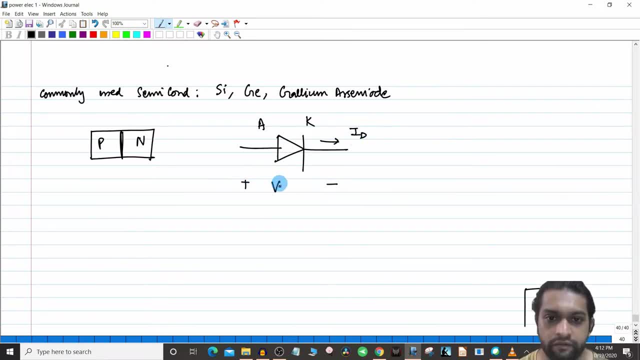 id. okay, and here you are having the voltage across the diode vd. so if the vd, if the diode is forward by the current, will move from left to the right side or in this direction, this arrow direction, i'll just draw it in it, i'll just color it little bit. so the arrow direction shows the direction of. 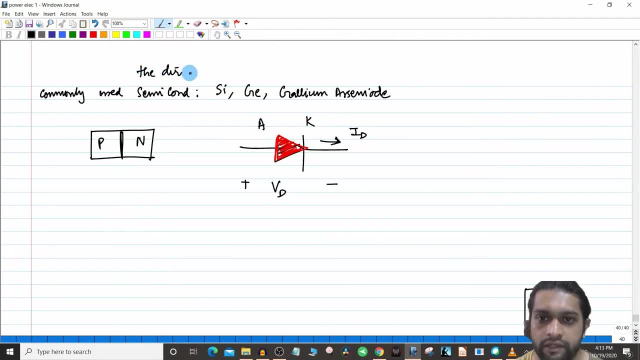 the current. the direction of the arrow. direction of the arrow shows the direction of the forward current. forward current. forward current is the current which is flowing when the diode is forward biased. okay, now it is simple. uh, when the anode is positive, the anode is positive with respect to, with respect. 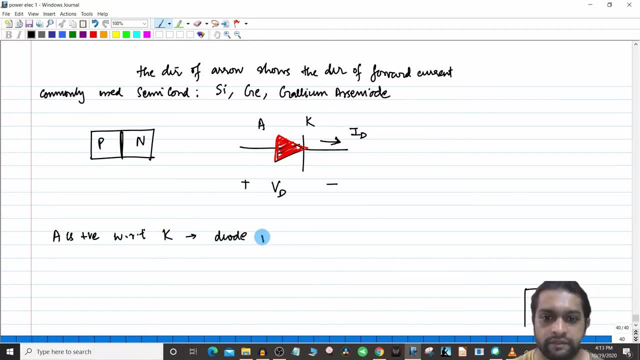 to the cathode. you call that. the diode is forward biased right. the anode is positive with respect to cathode, the diode is forward biased right. and what happens then? it starts conducting, the diode starts conducting and forward current flows and the forward current flows, forward current flows. 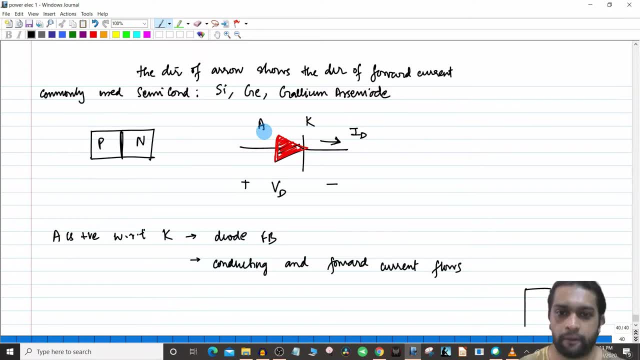 now, inside this diode itself you will have a small voltage drop. that voltage drop is called the forward voltage drop of the diode. the diode has a small voltage drop. diode has a small voltage drop across it, which is called the forward voltage drop of the diode. okay, so usually that ranges. 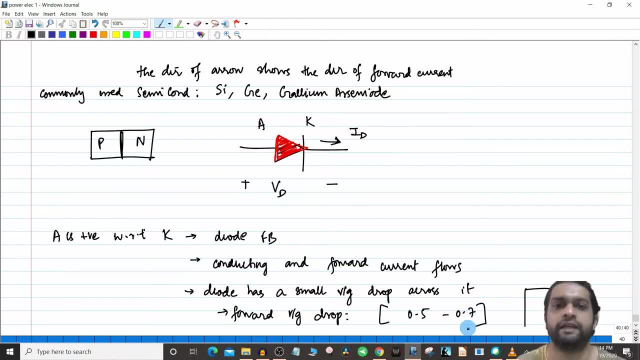 from 0.5 to 0.7 volts, depending upon the material of construction, depending upon silicon, depending of germanium and depending of gallium arsenide. it can have values from 0.5 to 0.7, usually numerical. they will give this value of what value you have to take to solve the. 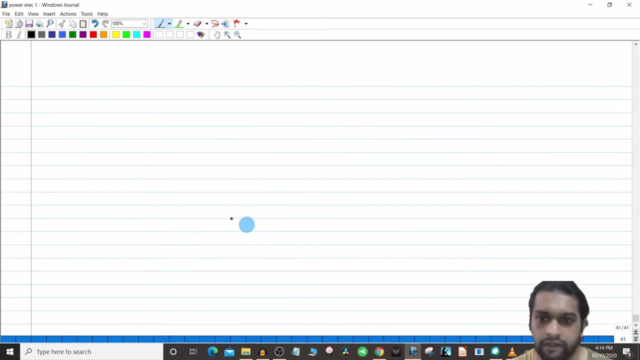 mistery, okay. similarly, if the anode is negative with respect to cathode, right, so here, anode, cathode. now the anode is negative with respect to cathode, the diode is called reversed biased. diode is reverse biased, okay, or you can call that: the diode is turned off diode. diode is in its off condition. 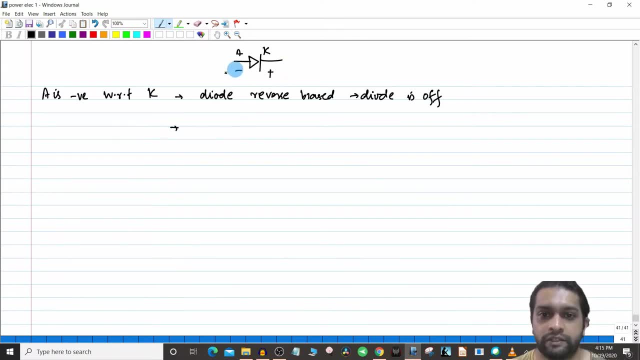 okay, now, in this case, what happens is that, because you are no device, that you will always have a current which is flowing, which is called a leakage current, and in this case, if you are giving a polarity like this, a small leakage current will flow. so a small current, a small current called reverse current, reverse current. 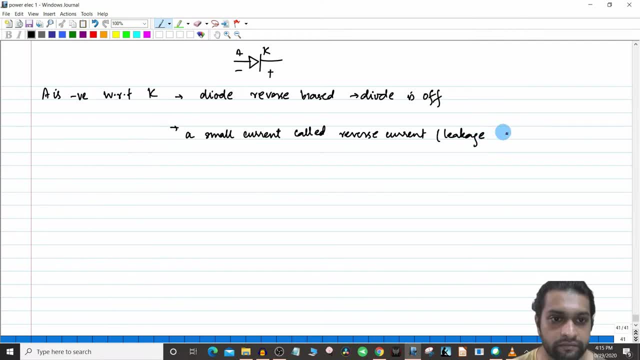 or the leakage current, or the leakage current may flow through the diode may flow through the diode. so what? all terms you have come across? you have a diode voltage. when you are putting forward bias, you are having forward current when you are putting reverse voltage. 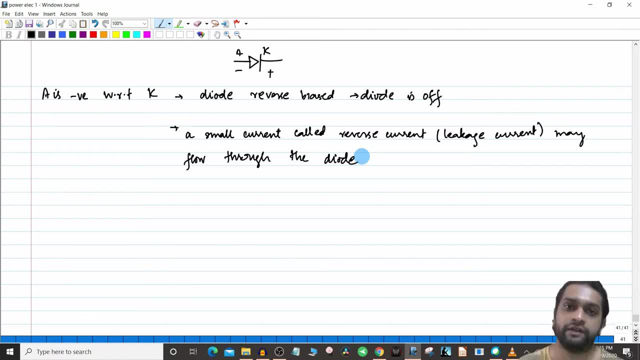 the diode is off at a small current, which is called leakage current or reverse current flows through the diode. okay, So now let us see. Let us just- I have just put up a small simulation. we will just see what, all terms- we have seen. 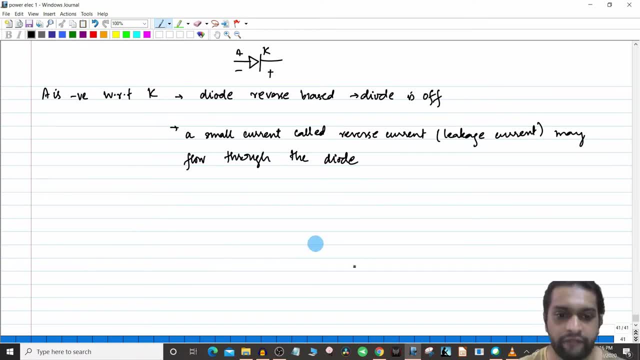 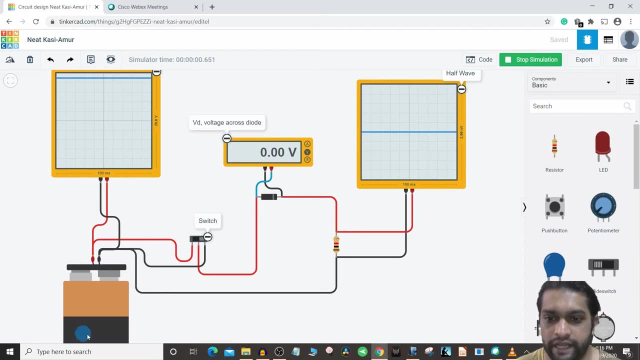 now here. Of course I will not be able to show the leakage current here, that we will see in an another video. So here you can see a small simulation which I have put up. So note here closely. So here is a 9 volt battery. this is a simple 9 volt battery. 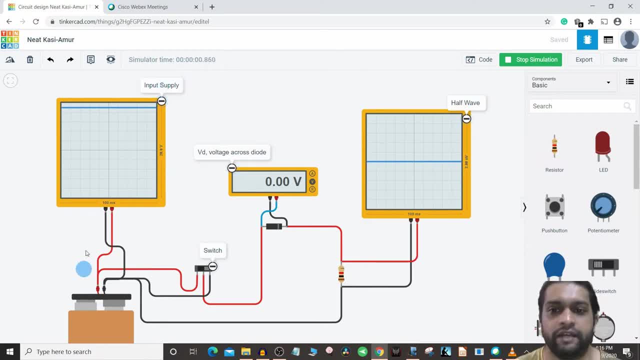 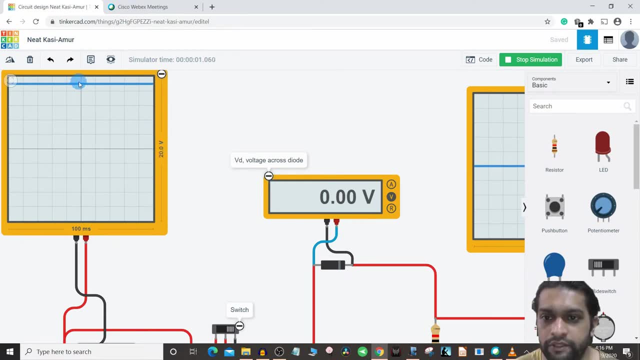 And this meter here measures the input supply, which is a 9 volt. So this, you can see that it is a 20 volt. this 20 volt from here to here, So from this point to this point, it is 10 volt. 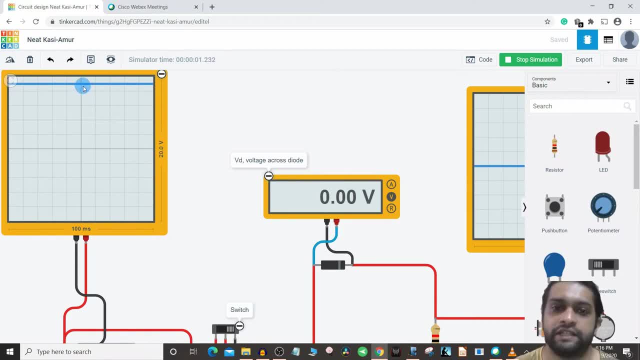 So each section is divided into five different divisions. So each division is 2 volts. So it is 2, 4,, 6,, 8 and 10.. So 9 volt is somewhere in the middle here. 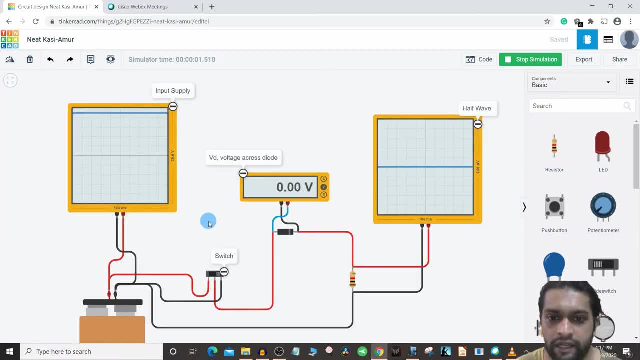 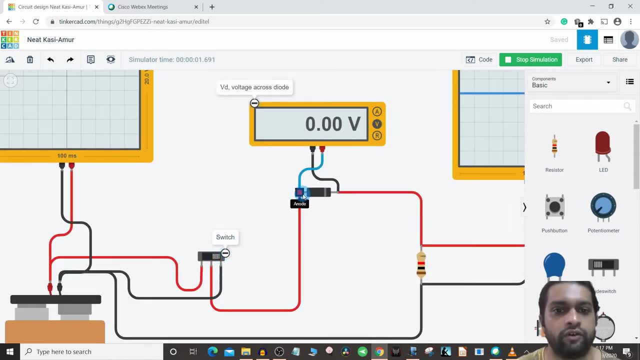 So between 8 and 10, you are having the 9 volts. So here you have a switch here. So at this point of time, in this position, in this position, the switch is giving 0 volt here. 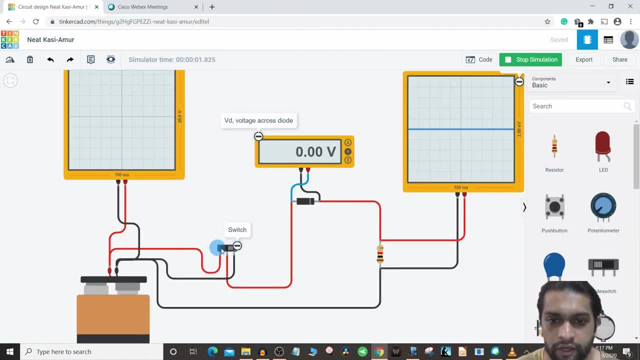 Switch is giving 0 volt to the diode. If I switch the, if I put the switch in the another position, You will get the 9 volt which is going to, which will apply the positive volt to the diode here. 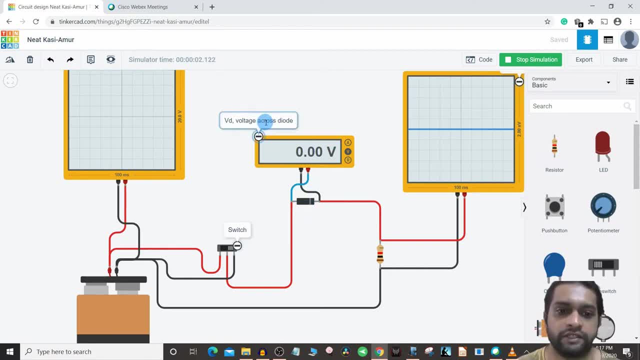 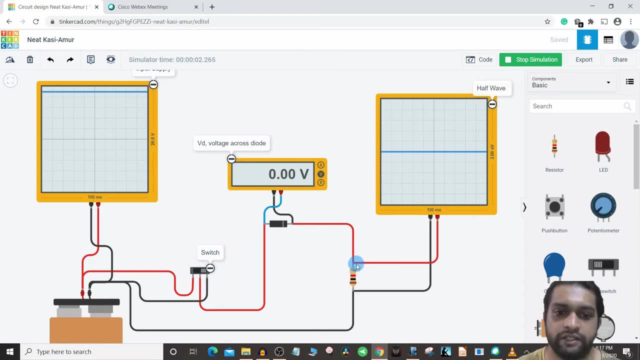 So this is the diode and this meter measures the voltage across the diode. Then I have kept a simple resistor here And this will measure the. this oscilloscope is going to measure the voltage across the resistor here, So I already started the simulation here. 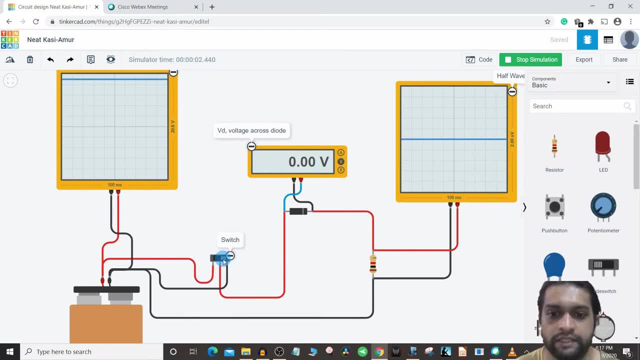 Now, at this point of time, at this point of time, this switch, switching position, I am applying a ground potential to the diode. Therefore, the diode is not working, The diode is not conducting, The diode is not forward biased. 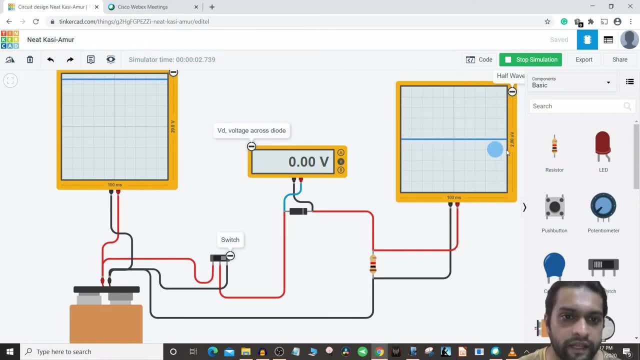 Therefore, if you see the output voltage is 0, right, the output voltage is 0. If I am turning on the switch, if I give positive voltage here, the diode will conduct and this output voltage will come across, this particular voltage. 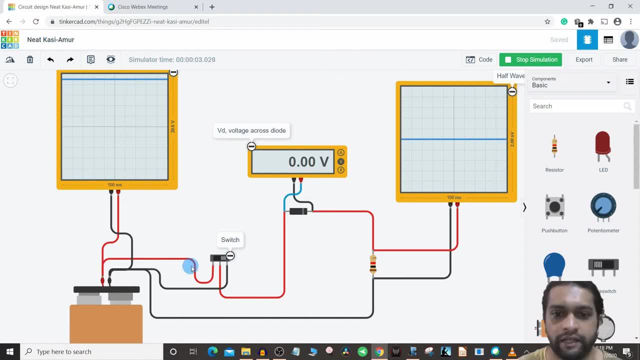 So this is 9 volt. So here also you are expecting 9 volt to come. right, The diode will conduct, the diode will conduct and this voltage will come here. So we will switch. So now I have switched, I have given the switching action here. 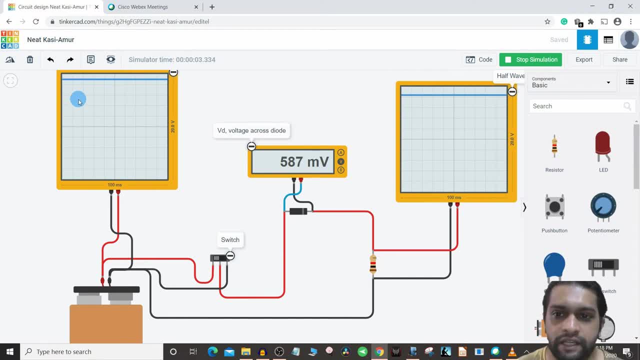 So it will take a little bit of time to stabilize. Yeah, So if you see here this is 9 volt, look closely. this is 9 volt here, but this is not 9 volt. It is a little bit less than the 9 volt. 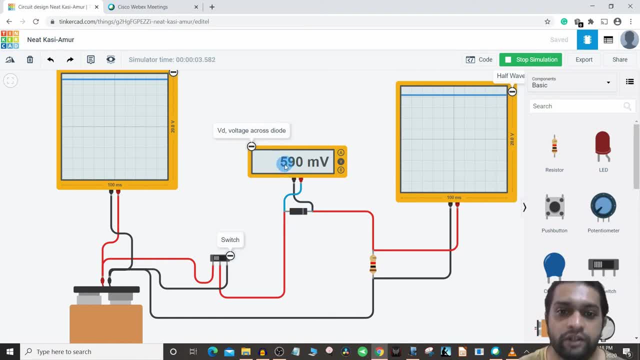 Why that happened? Because when the diode is conducting, there is a voltage drop of 590 millivolts or 0.59 volt or 0.6 volt across this diode. So this 10 minus this 0.6 volt or 0.59 volt will come across the load voltage. 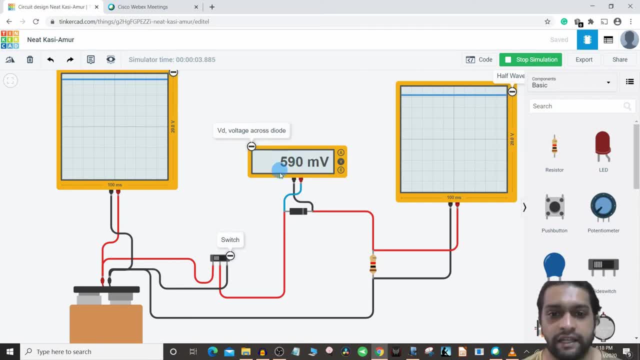 So that is the idea here. When the diode is conducting the forward direction, there will be a voltage across the diode, But in this case I am not showing the reverse leakage current here. That we will see when we do a more detailed simulation. 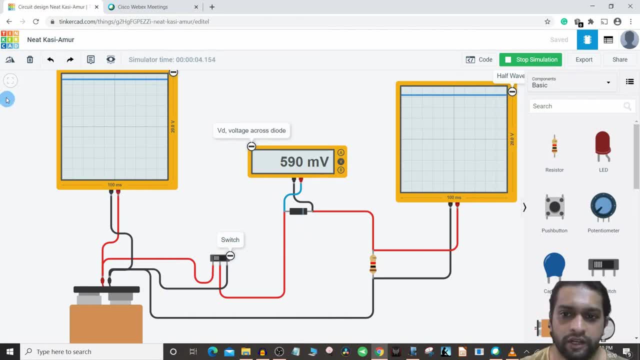 So here we are just trying to see all these things. So this is not a rectifier circuit Here. this is a very simple circuit. I am just switching on the diode using a positive voltage. This is not a half wave or a full wave rectifier. 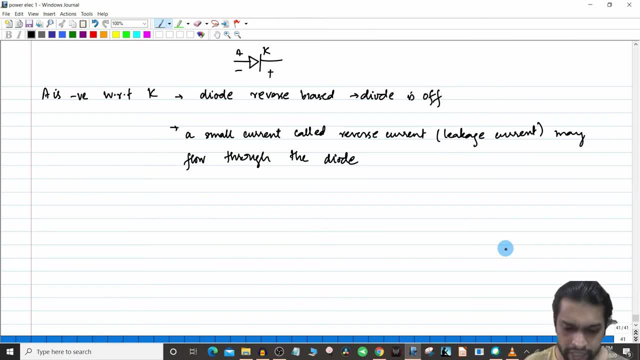 That will come in the later part of the videos. Okay, This is what we have seen in this particular video. Now, if you draw the characteristics, that is the characteristics in the sense, if this is the diode, So this is the anode. 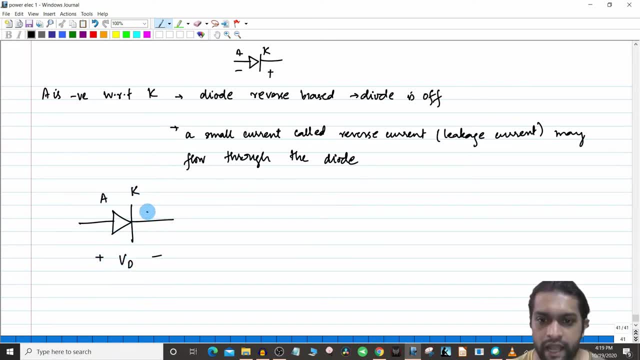 This is the cathode, This is the positive voltage, Vd, and this is the positive forward current, Id. So in an ideal diode, what will be the characteristics? In an ideal diode, even if applied, very, very less voltage should be applied for the current. 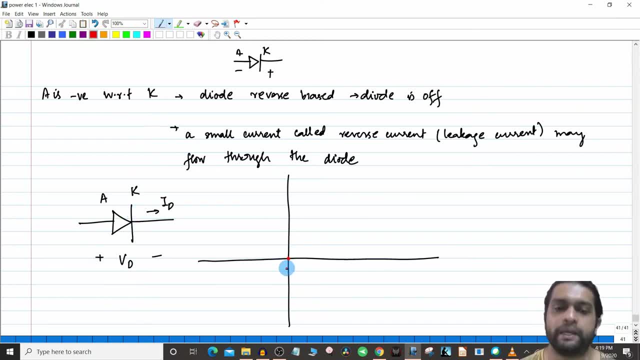 to flow. That means, in an ideal case, almost a 0 volt current, So 0 volt should be applied. This is Vd, this is Id. Even if a 0 volt is applied, the current should increase. So this will be the characteristic. 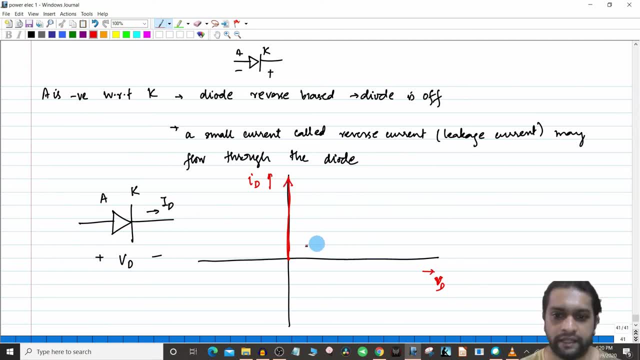 And in an ideal case, how much ever reverse voltage I apply, that means this is positive voltage Vd. If I apply a negative voltage Vd, so this is negative voltage Vd. how much ever negative voltage I apply, the current should not flow. in an ideal case, 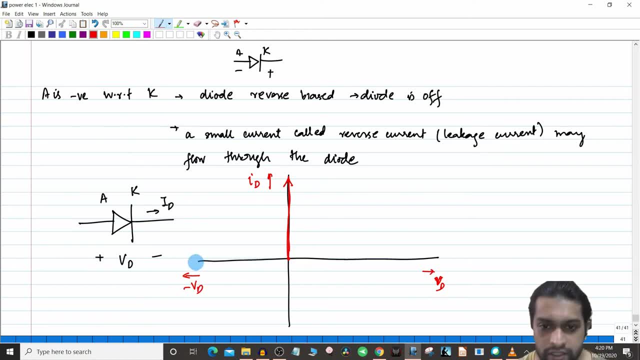 So if I, whatever voltage I apply in this side, whatever Vd value I apply in this negative direction, it should not give any current. So in the ideal case it should be like this, But you know that all cases are not ideal. 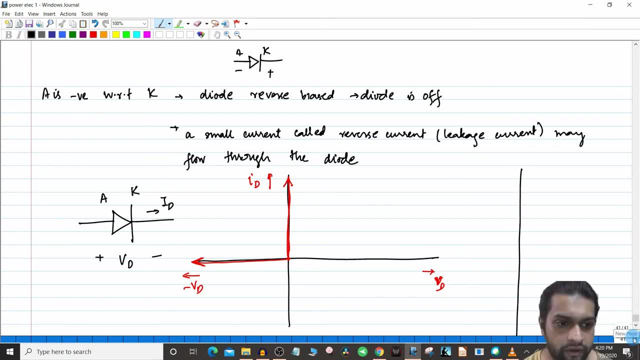 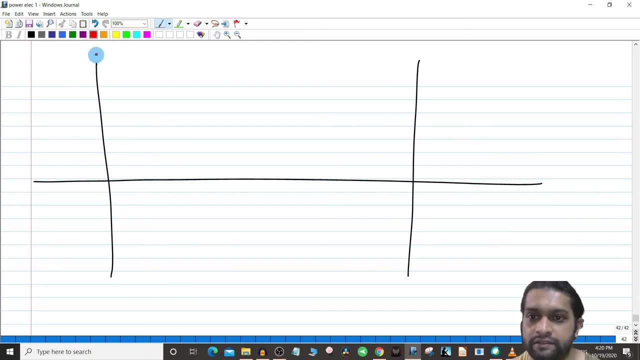 We are talking about practical switches now, So we will draw it in next page. So, in the ideal case, we will just draw it everything very fast. So this is ideal case. So this is ideal case. So this is Id, this is Vd, Id and this is Vd. 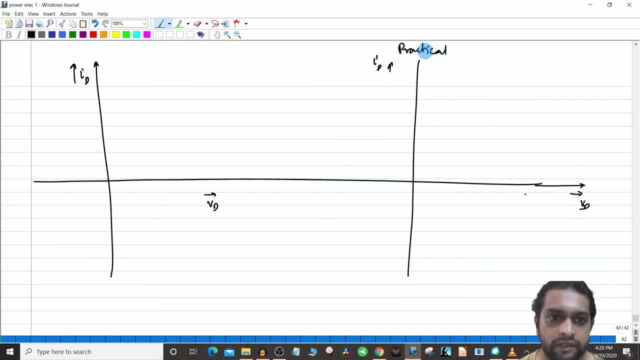 So this is for practical switch and this is for ideal diode. So you saw that in the ideal case the characteristic look like this, But in the practical case you know that the current will start to build up only after this 0.6 volt, because 0.6 volt itself is dropped across the diode. 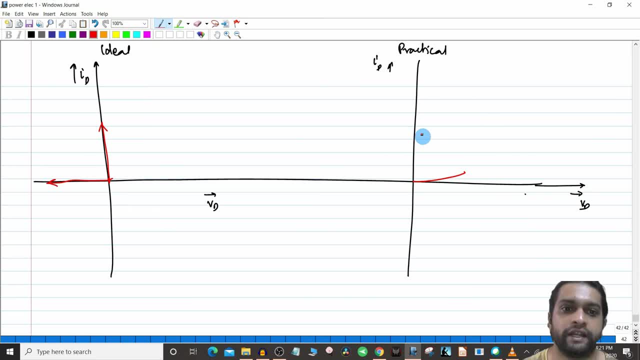 So the characteristics look something like this: Till this point you won't get much increase in current, But after a particular value, which is also called as Vt for a threshold voltage, the current starts increasing rapidly. The current start increasing rapidly. 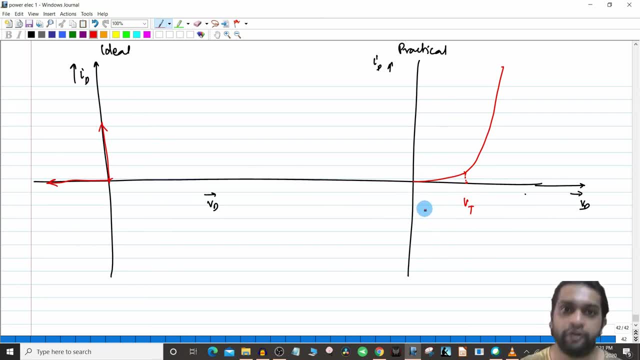 So after this particular diode voltage, after Vt, This is not supply voltage graph, This is the voltage across the diode, though it is not that 9 volt, This voltage across the diode. After that point, 5 or 0.7 volt across the diode, the current will increase rapidly from. 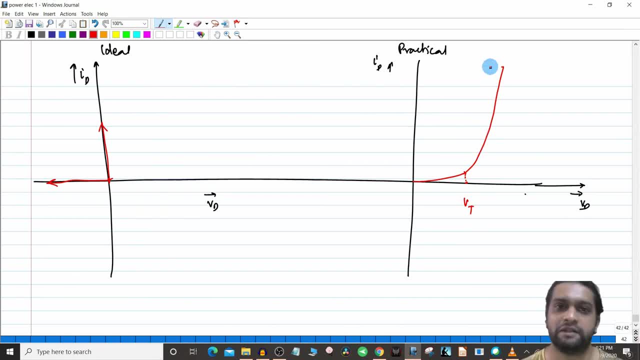 the current rapidly depending upon the. do not think this current will go to infinity. it will be limited to the value of resistor which you have or value of load which you have applied. ok, That we will see in the later class. So this is minus Vd. So in the ideal case, you saw, 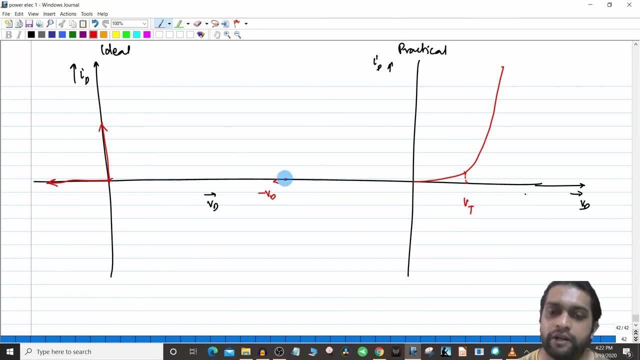 that whatever negative voltage you apply here, whatever negative voltage you apply here, there will be zero current, but there will be always a reverse leakage current. So when you increase the negative direction like this, there is a small amount of current. that is. 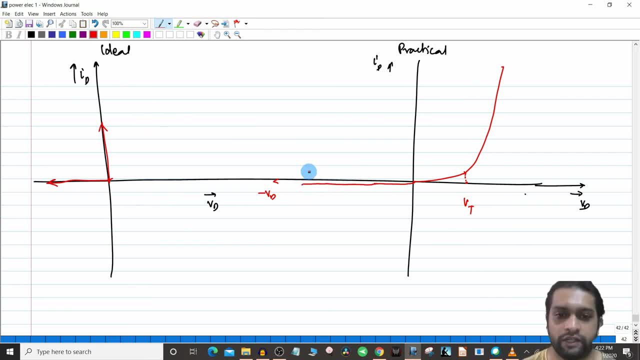 flowing and after a particular voltage, which is called as a breakdown voltage, the current will start increasing rapidly. ok, You might have already learned this. This is also called as the Avalanche breakdown. Now, if you see, here the current is constant. There is a 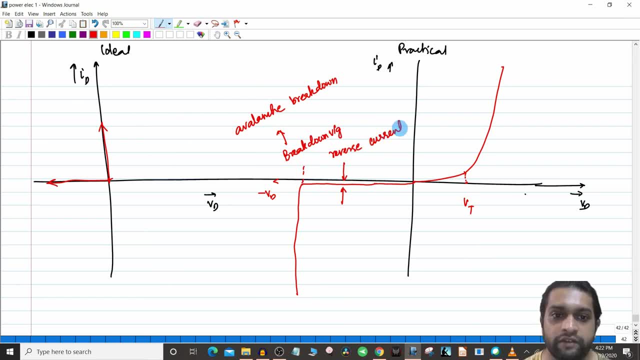 current is constant irrespective of the voltage which was I was applying. reverse current was constant irrespective of the negative voltage I was applying. that is because, actually, the equation, the diode equation, which is popularly called, is also called as the Shockley diode equation. Shockley diode equation. Id is equal to that is, the diode current is equal to Is. 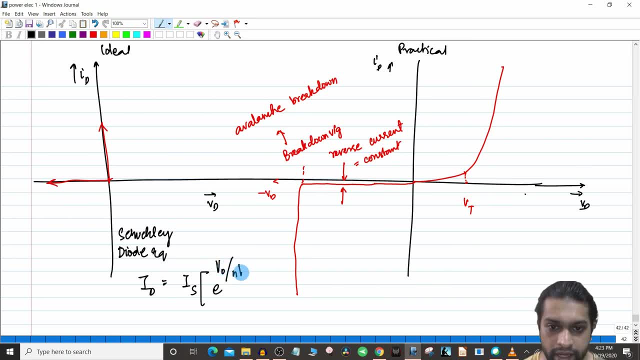 into e power. Vd divided by n into Vt minus 1. in the next video we will go through this equation in a much depth manner and we will see why this reverse current is constant. so I hope today you have liked this video. so till I say in the next video is me Varun signing.